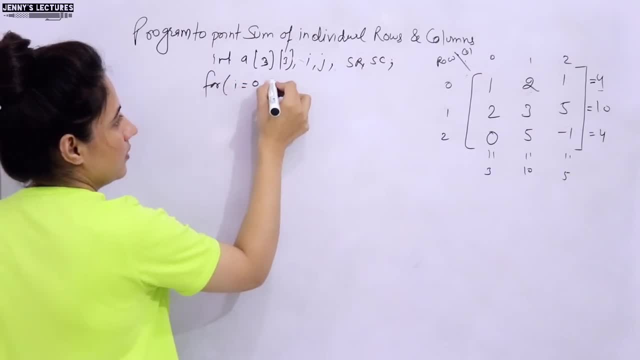 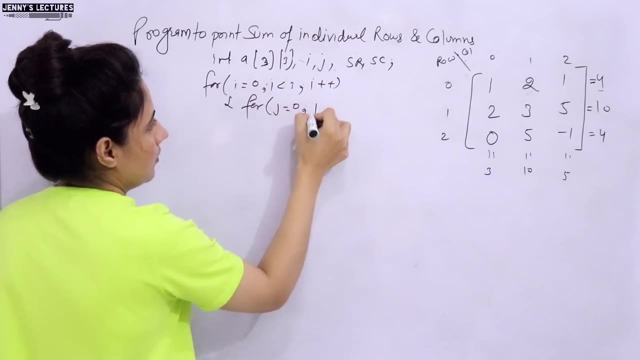 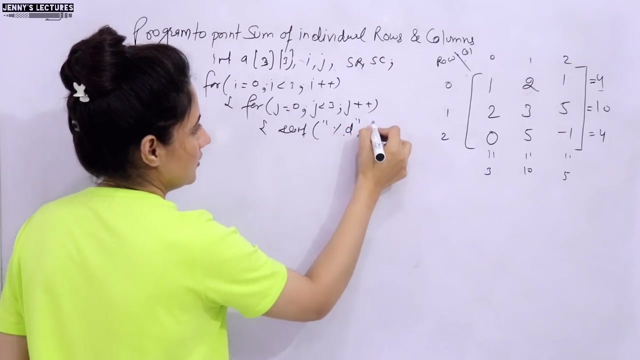 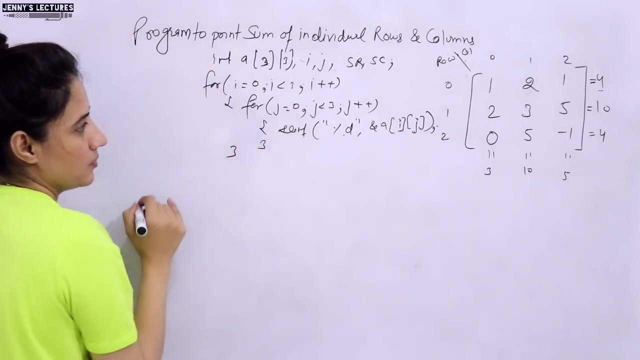 Now input. Or you can say: read this matrix. I hope everybody is clear with this syntax because we have used this syntax many times. right, i and j. scanf i and j. This has to read the matrix 3 into 3 matrix, 3 columns and 3 rows right. 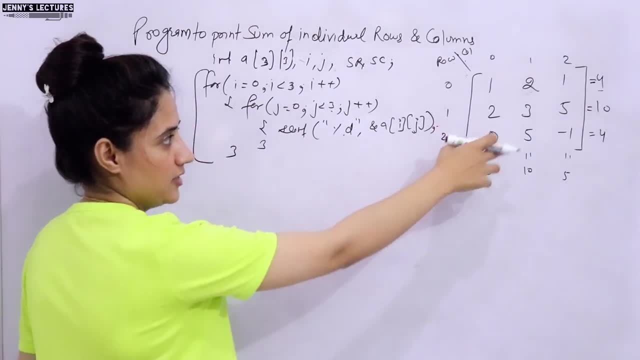 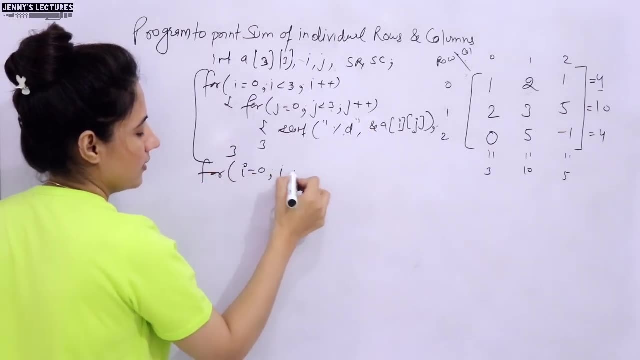 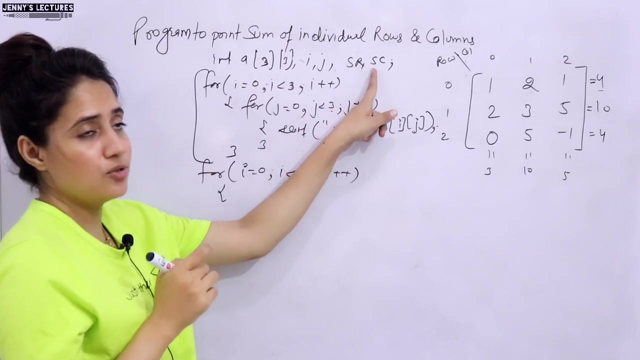 Now we will access the elements and as well as we are going to print the sum right. So obviously 2 for loop, i should be 0.. i less than 3 and i plus plus right Now. see, I have not initialized these to 0. And previous videos I have told you you have to initialize the sum to 0, otherwise it will take any garbage value. Why? 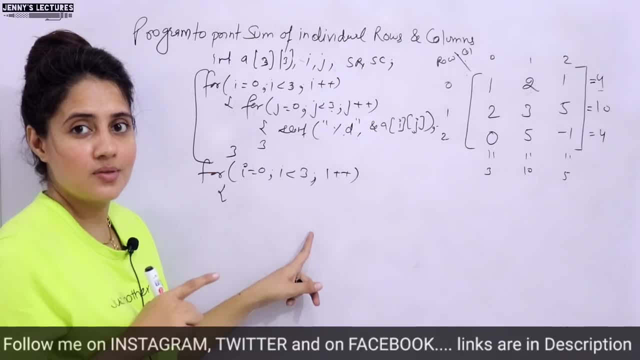 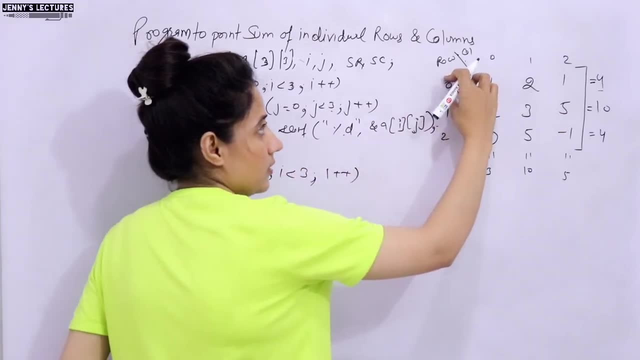 Because I am going to initialize it in this 4 loop, Because I am going to print, I am going to sum the individual rows. So, after sum, after doing sum of this row, right, that is 4.. Right, That is 4.. 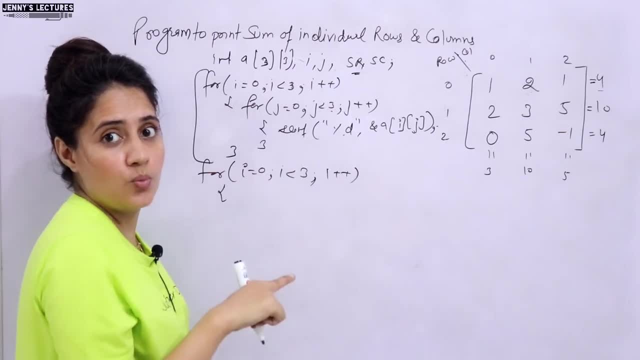 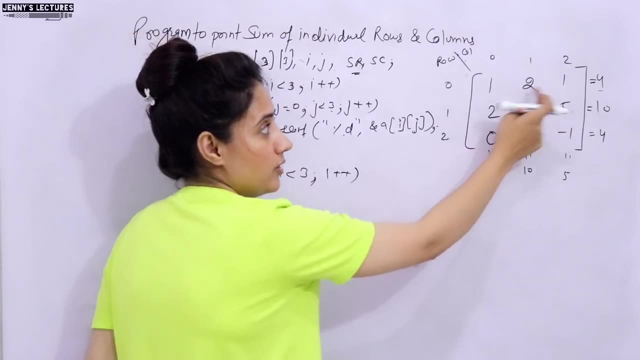 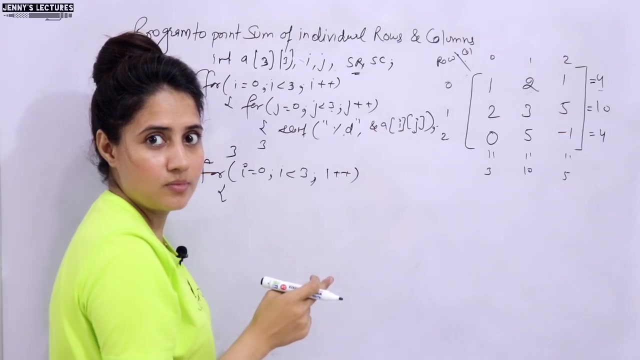 sum of r variable should again be initialized with a 0 for this row. Otherwise, if you will not again initialize it with a 0, then it will do what For sum. for first row it is 4, then in 4 only it will add these values. Maybe you are not getting this point right now, but 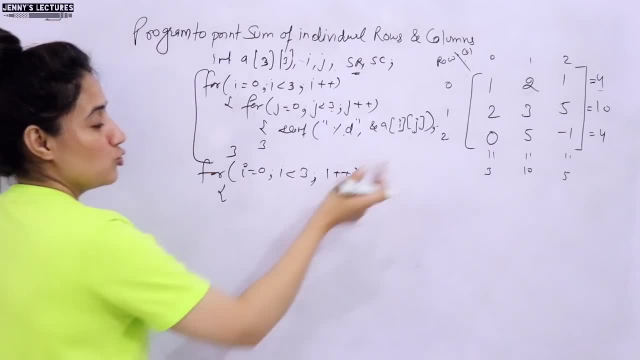 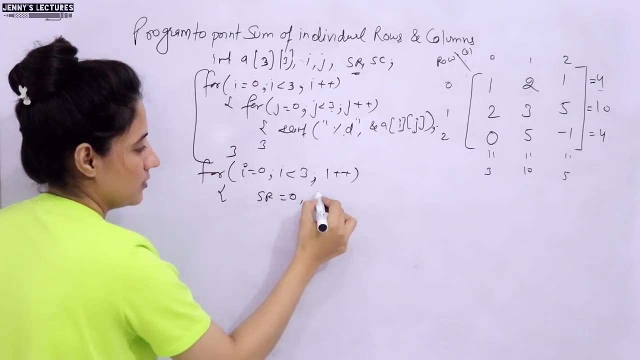 it is ok, I will try run this program then you will get it better right? So where we will initialize these sum within this 4 loop? right? sr 0 and sc is also 0, right? or you can initialize something like this: sr equal to sc is equal to 0. right Now, another 4 loop. 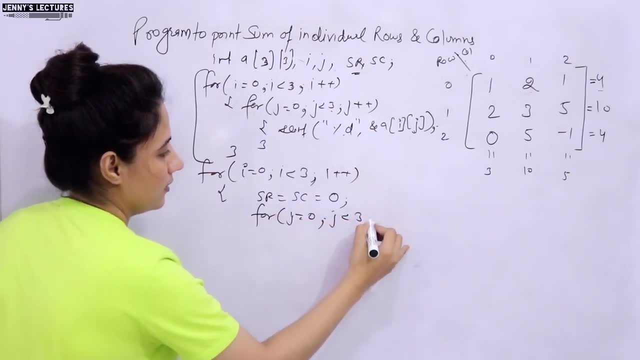 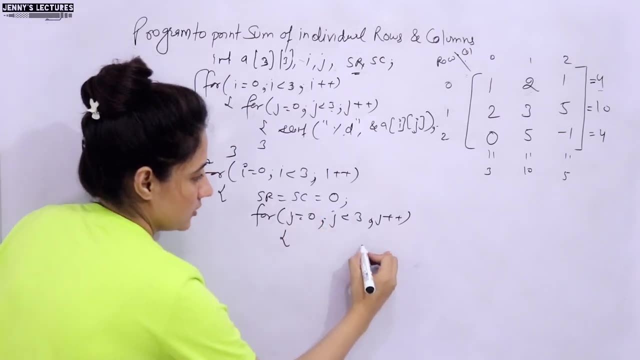 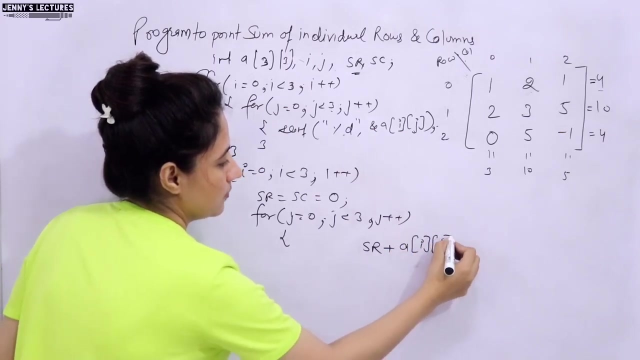 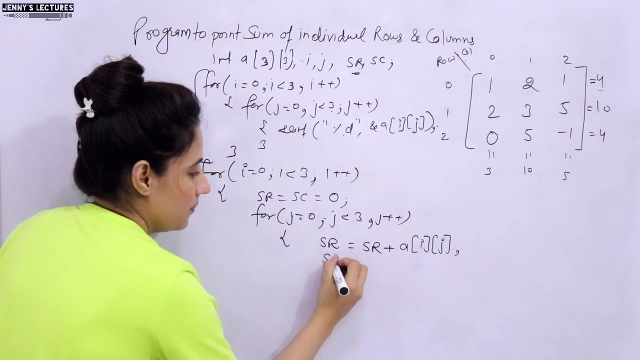 j is equal to 0 and j less than 3 and j++. Now in this 4 loop we are going to do sum right, So sum of rows, sum r plus a of ij, and that would be stored in sr right and sum of column. 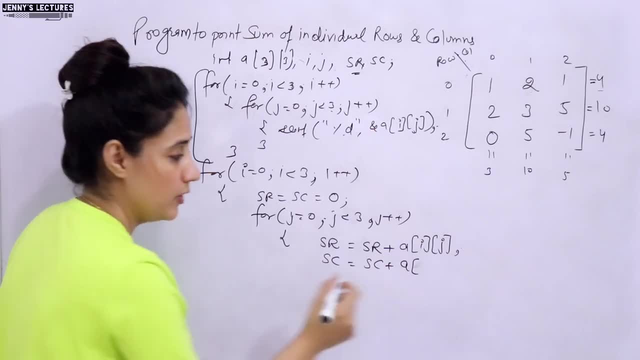 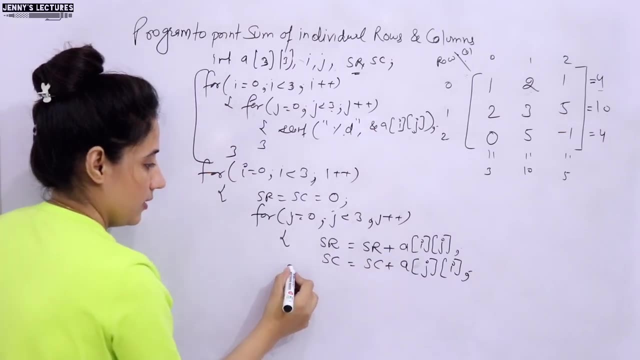 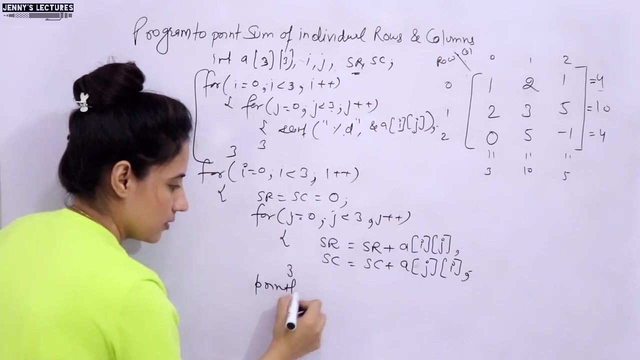 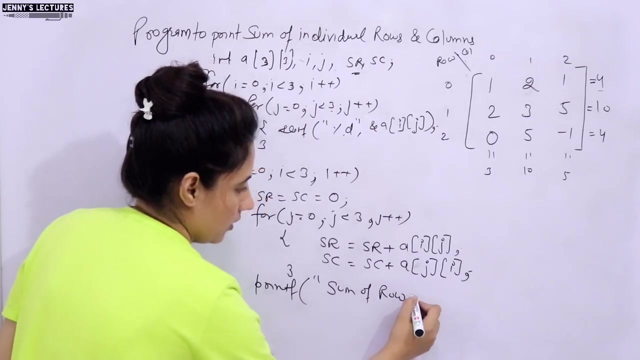 sc plus a of. Now for columns, we will do what ji, we will interchange it right, and that is it. So after this 4 loop, after this inner loop, we are going to print Sum of row. or you can say: rather than writing this small, I am writing sr equal to percentage. 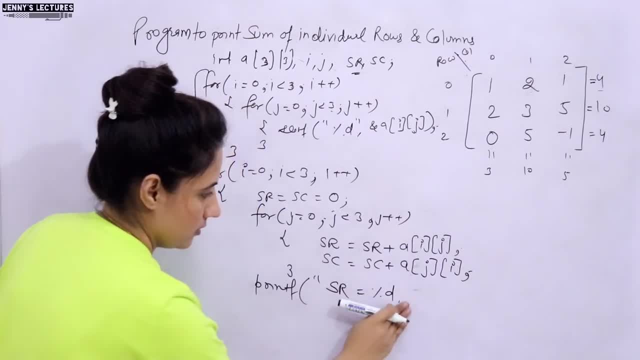 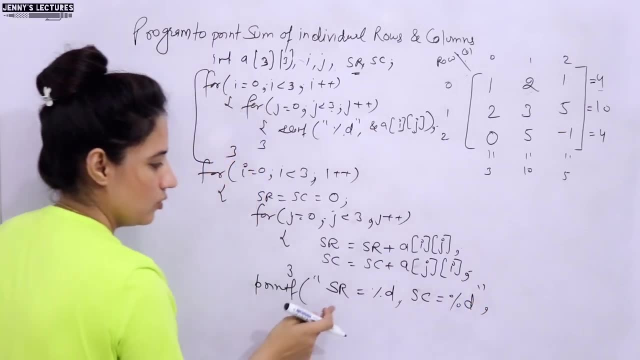 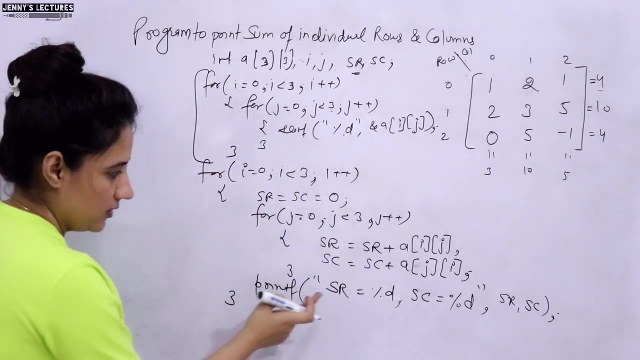 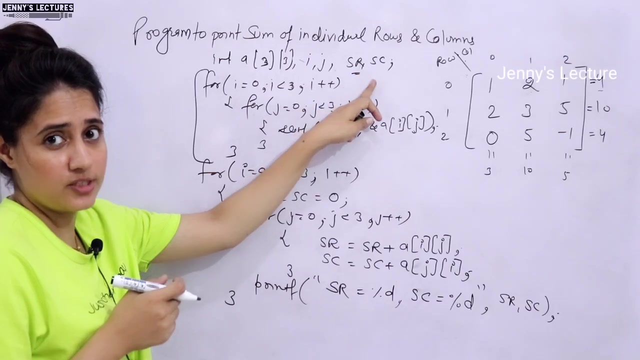 d and, sorry, sr comma sc, equal to percentage d, in one line line only. I am printing both, the sum S R comma S C, right See, I am taking this S R and S C like in capital letters, just to make you understand, like, and these are sum of rows and sum of columns, But according 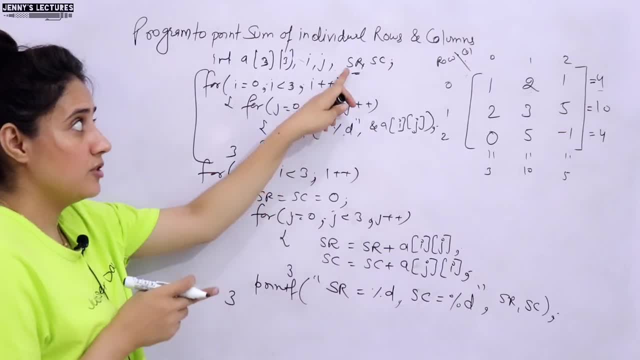 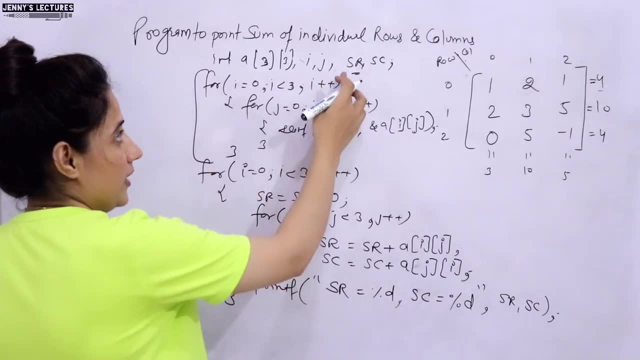 to the naming convention of that variables. you can take it like first variable. first, you know that letter of this should be small. it is better to take small, So you can take it in small letters also, right. or you can take it something like this, like sum and S. 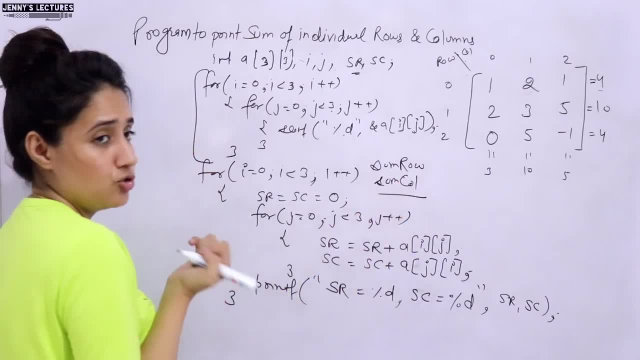 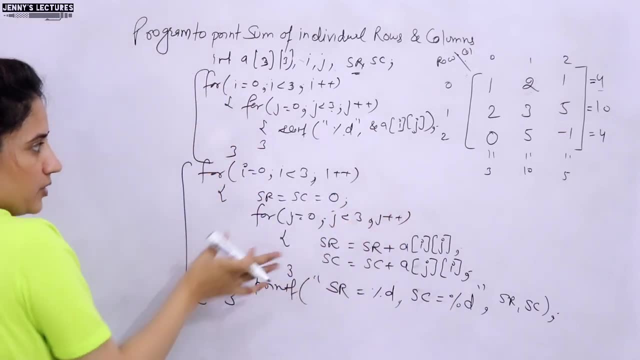 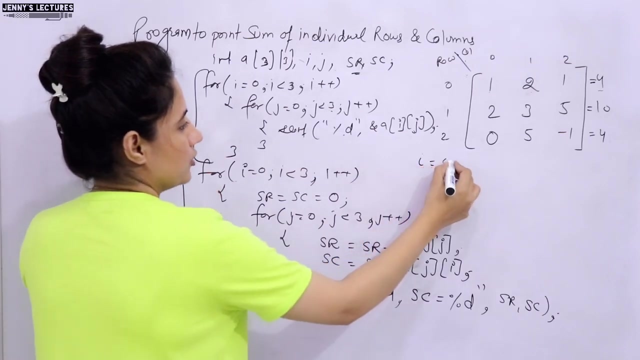 comma, row and sum and column like this you can also take right Now. let me just dry run this program for you, then you will get the working of this 4 row right. See, this I hope you got. I have entered this one right Now. see, I value is 0 fine. 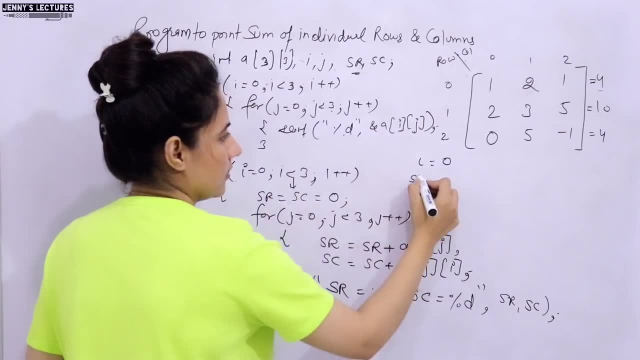 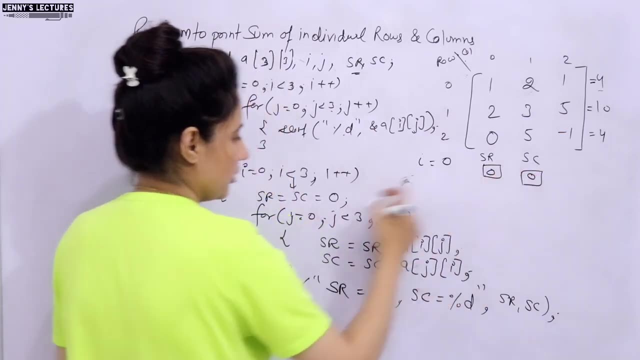 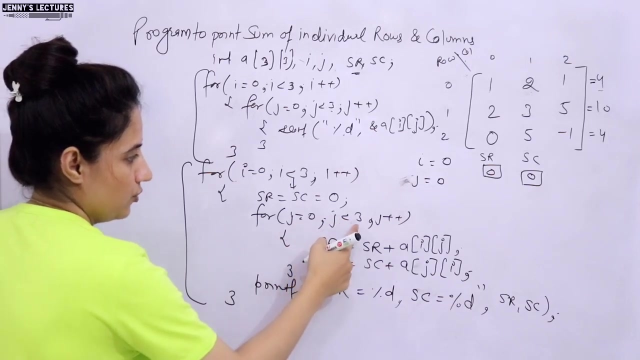 I less than 3? yes, condition true: enter here Now S R S R and S C S R S C. both are 0.. Initialized with 0 within this 4 row right Now. J is also 0.. Condition: true: yes, again. 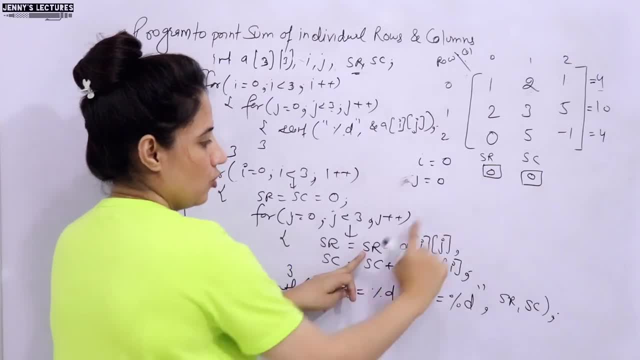 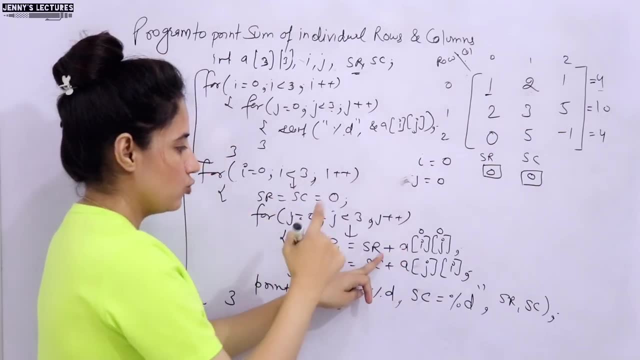 enter here. Now see S R plus A of I J. S R is 0 plus A of I J. I and J. both are 0. A of I J means this thing: 1.. So 1 plus 0, that is 1 that would be given to this S R. that. 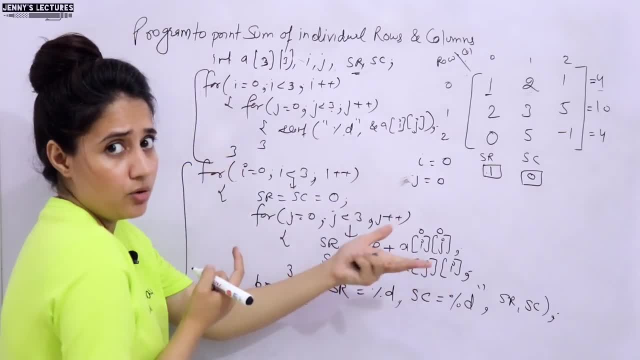 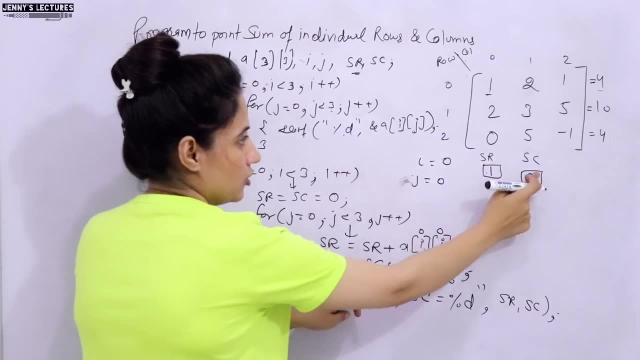 is 1.. Now S C plus A of J I. Now both I and J are equal. that is 0: 0.. Same variable. we will access 1 and 1 plus S C is 0 and again it will become 1, right. 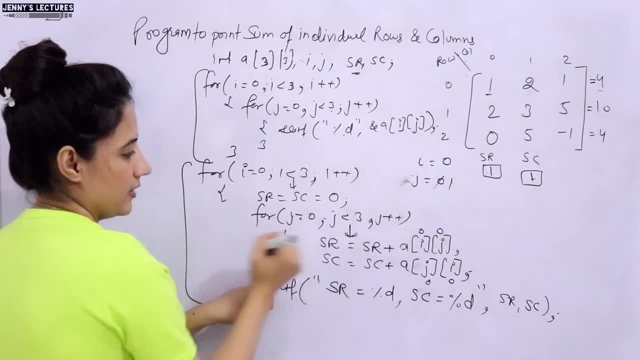 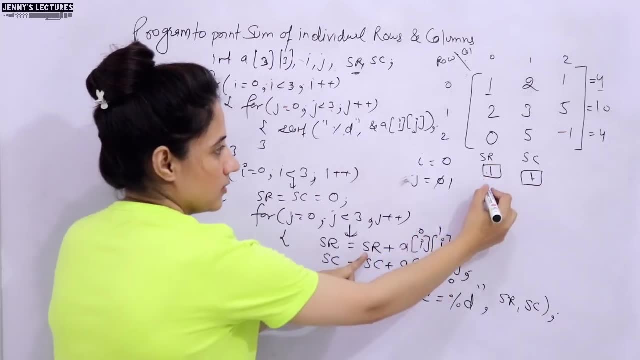 Now we are in this inner loop. Now J plus plus J becomes 1.. Condition true: yes, again, enter here. Now S R plus A of I, J, J is now 1.. Now S R is 1 plus A of 0, 1.. 0, 1 means this: 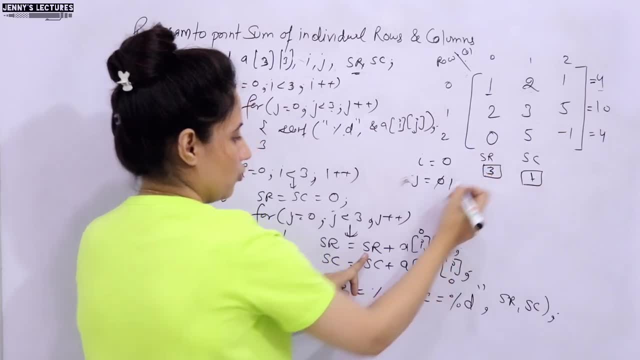 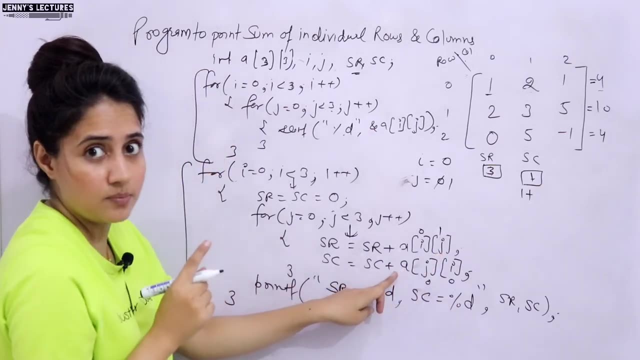 one, 2.. So 2 plus 1, 3. So 3 would be assigned now to S R. Now S C plus S C is 1, 1 plus A of now J. I See it is for column right. So that is why means we are accessing, we have to access this. 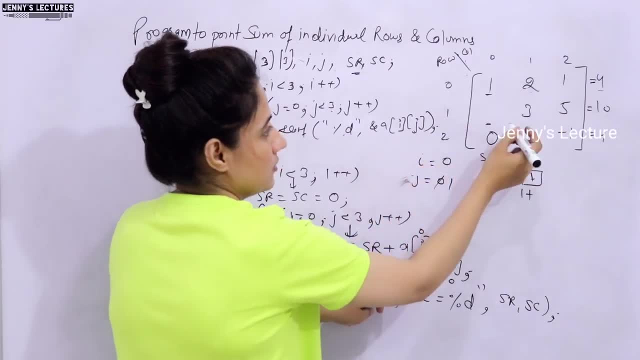 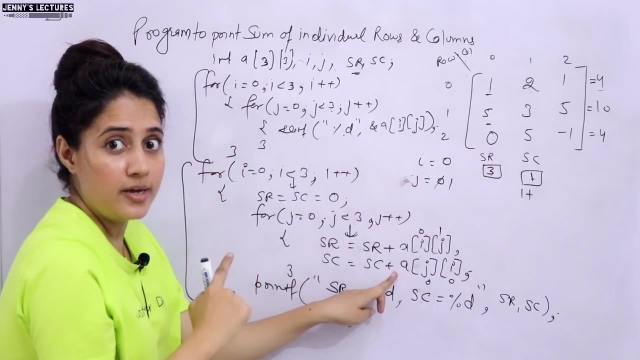 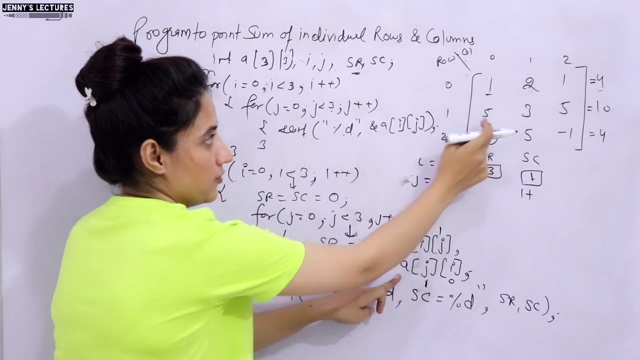 2, right, or let me just change it? I am just doing it. what 5.. So now we have to access this 5 for this column. that is why I have interchanged: rather than I J, I am taking J, I. So now J is 1 and I is 0.. 1, 0, 5, this element 5.. So 5 plus 1, that is 6, and now S C becomes. 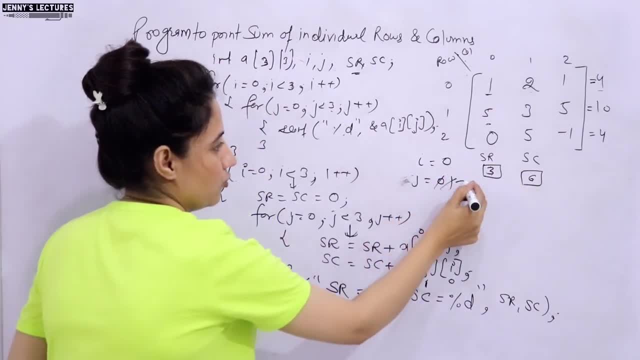 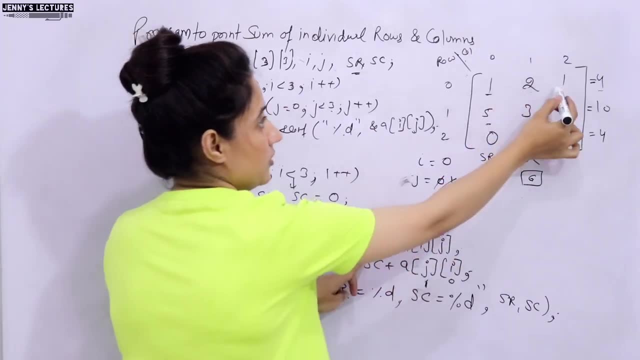 6. right Now again. J plus plus J becomes now 2.. Condition: true: yes, enter here. Now. S R plus A of now J is 2. 0, 2. 0, 2 means this one, So S R is 3. 3 plus 1, that is 4. S C plus A of now J. 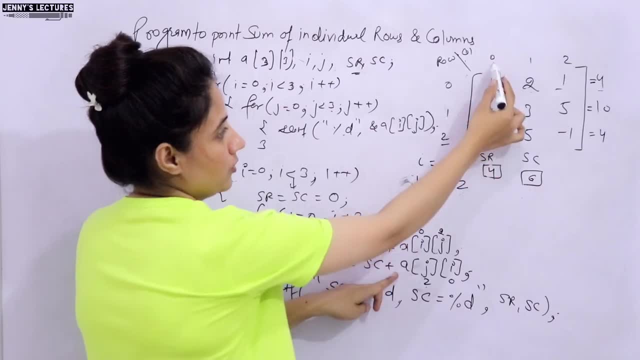 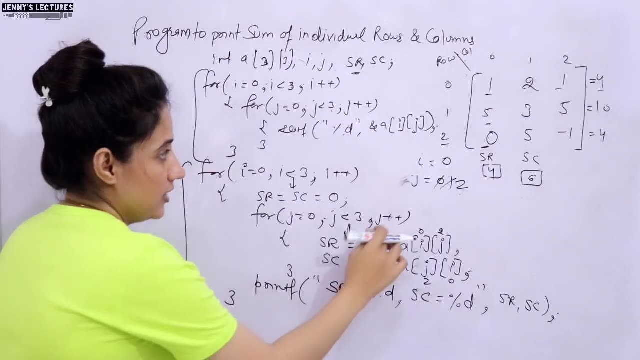 is 2.. 2, 0.. 2- 0.. This variable you want to access, that is 0.. So value would be same: 6. right Now again, J plus plus J becomes 3. but now condition is not true. 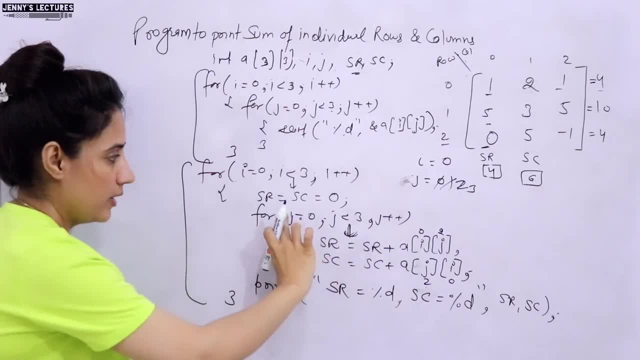 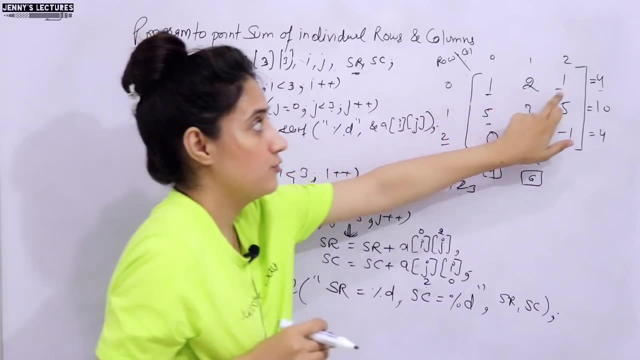 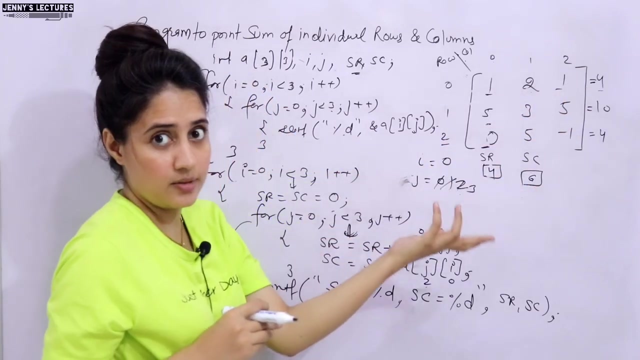 So exit from this inner loop and after this inner loop, whatever the statement that would be executed. So now here, obviously we have done sum of first row and sum of first column. This is 4, 2 and 3 and 4 and this is 6. yeah, So we have to print this one, 4 and 6, that. 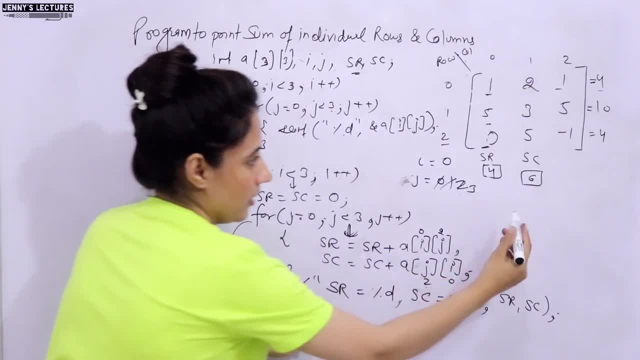 is why, within this for loop, outer for loop, I am printing, printing S R. now, output would be S R equal to 4 and 6.. Okay, Now, what do we get? How many columns are we going to get? 4 and 6.. Who will be in this? 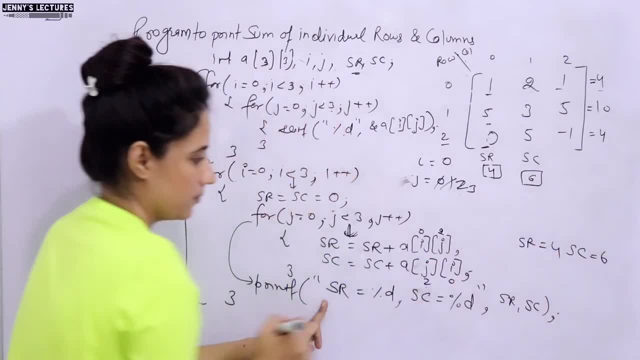 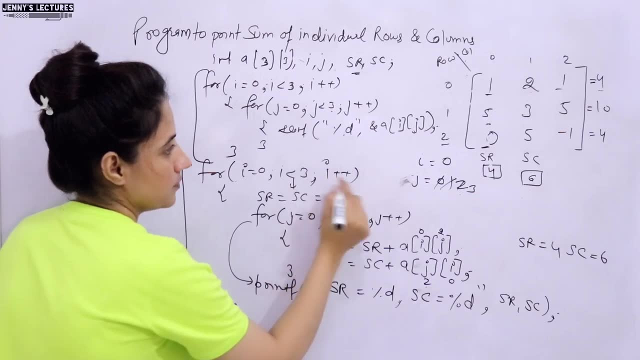 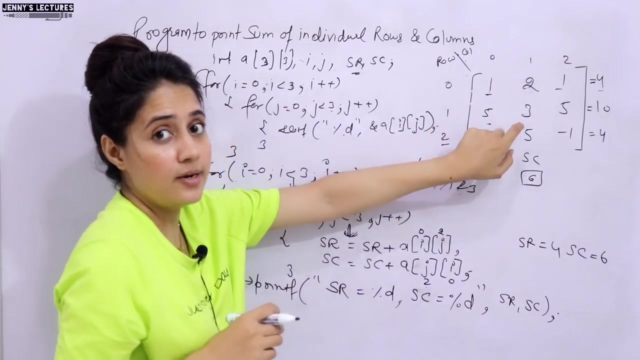 And SC equal to what, 6. That would be the output, Right, But still we are in this outer loop. So now I plus plus Now I becomes 1.. Right Now we want to sum of. we want that it should give sum of this row and this column second one. So that is why, again, we have 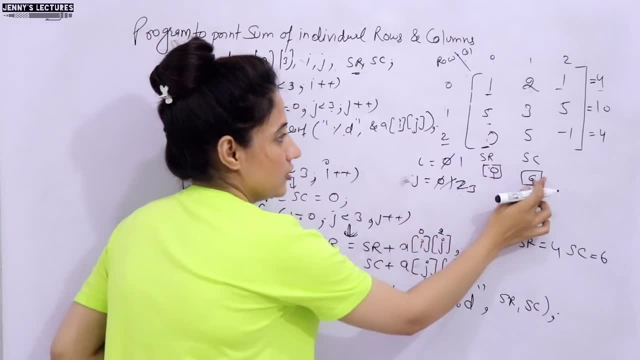 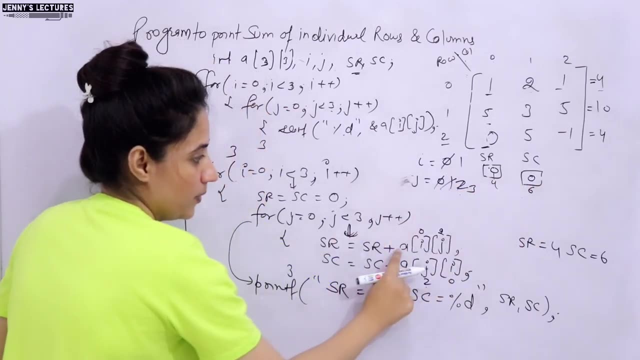 to initialize this SR to 0 and SC to 0. If you will not initialize, then it will take what 4 and 6. So 4 plus and 6 plus. So it will not give you correct output. That. 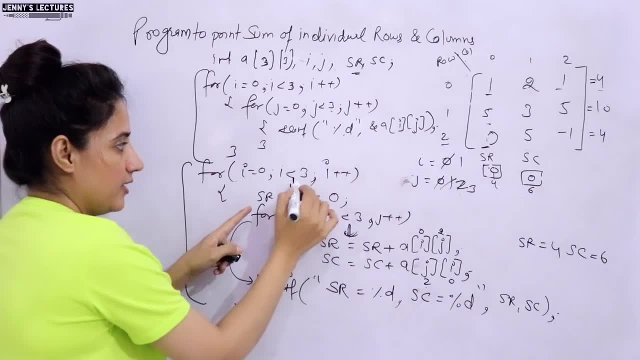 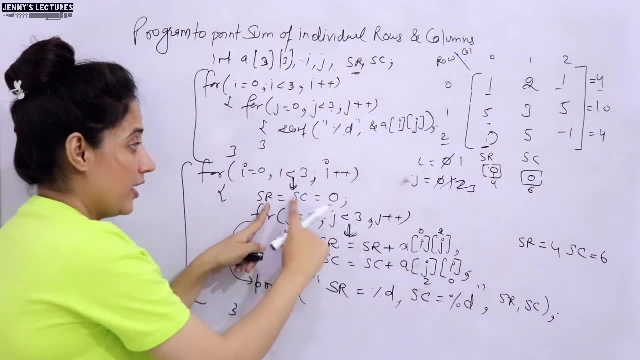 is why now I plus plus I 1 condition true again enter here Now. that is why I am initializing this SR and SC in this 4 loop, not here. I hope now you got my point. Now again, SR and SC are 0, 0. 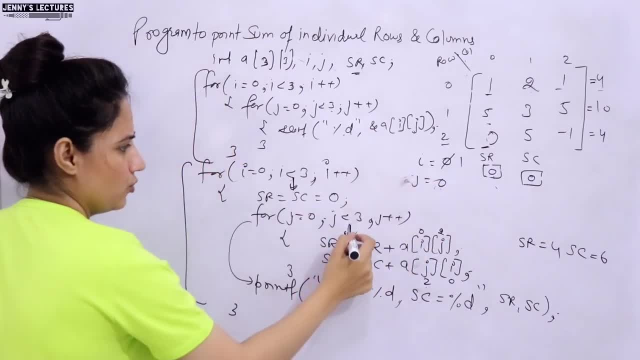 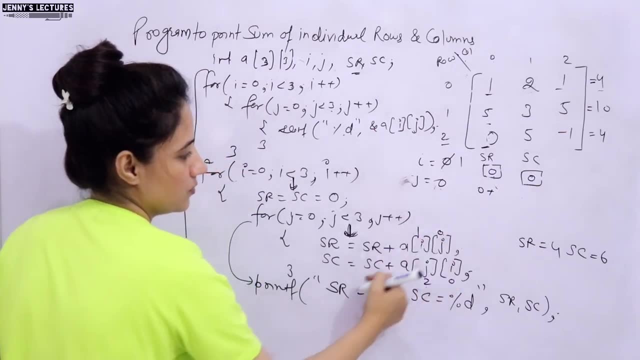 J. J is again now 0.. Condition: true again. enter here Now SR plus Now SR is 0 plus A of now. I value is 1,, J value is 0. So it will access 1, 0.. 1, 0, that is this one, 5.. 0 plus 5,. 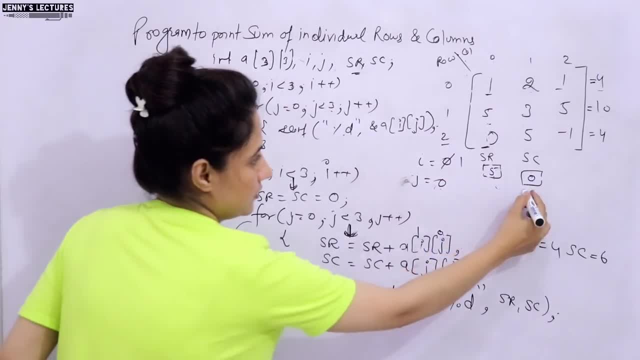 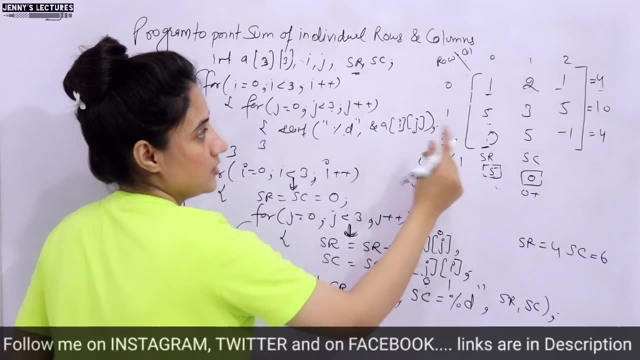 5. So it is 5. SC plus SC, 0 plus J is what. J value is 0 and I value is 1.. So it will access 0,, 1.. 0 and 1.. This one, This two. 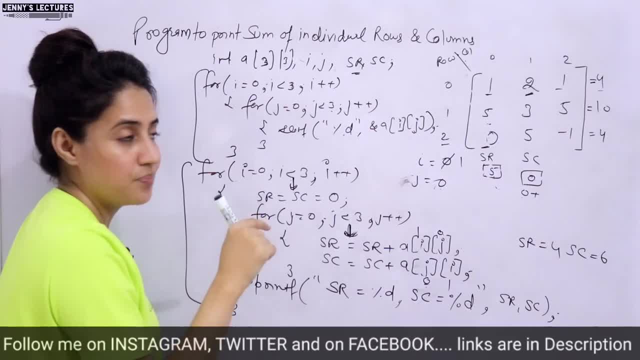 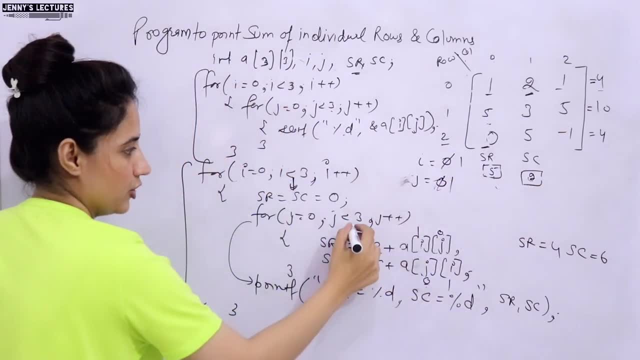 Because I want sum of second column, now Second row and second column. So now 0 plus 2 is 2.. Now J plus plus Now J becomes 1.. Condition true again, enter here: SR plus A of I is 1,. 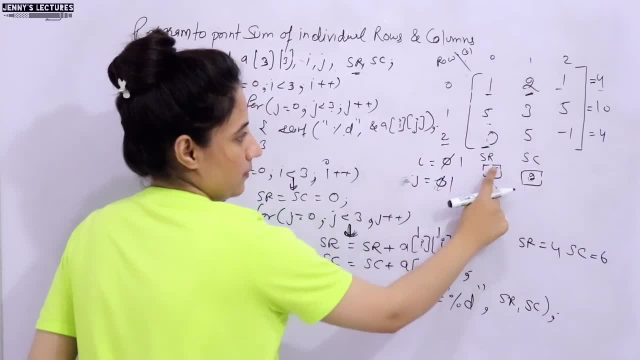 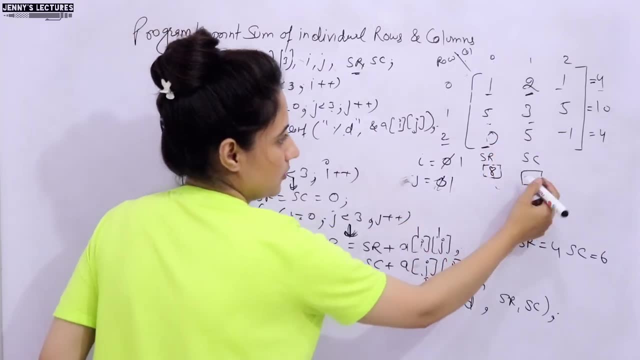 J is also 1.. 1, 1, that is 3, means it becomes 8.. SC plus both are 1, 1, that is this 3. So this becomes 5.. Again, it becomes 2.. Condition true: enter here SR plus. 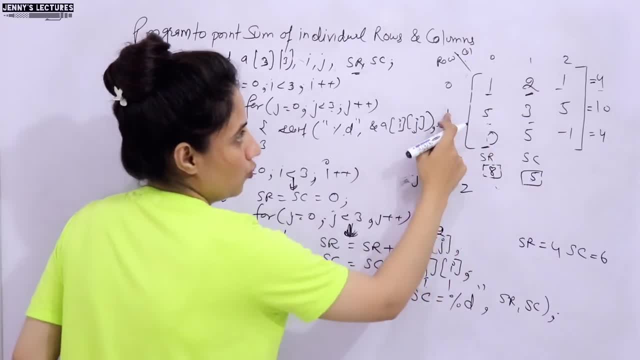 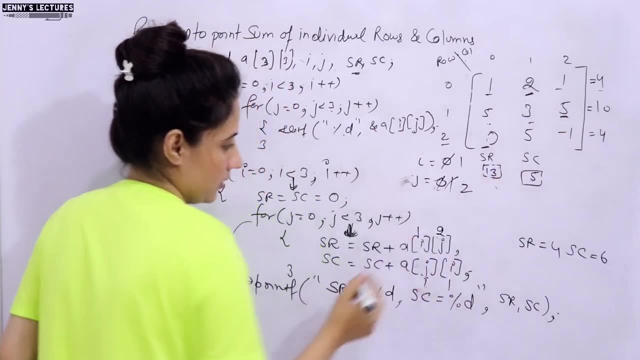 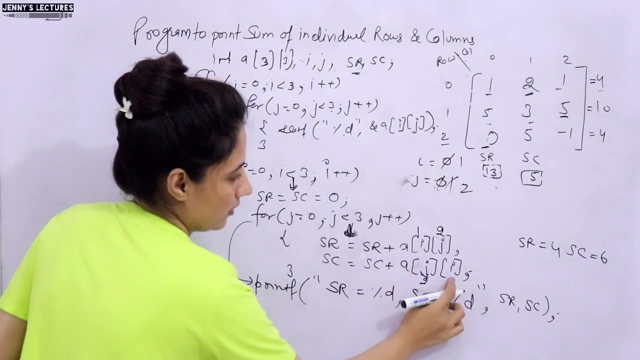 J of 1 and now J is 2.. 1,, 2.. 1 and 2.. This one, 1 and 2.. 5. 8 plus 5 is 13.. And SC plus Now J is what? 2 and it is 1.. 2, 1. Means 2 and 1.. So I want to access now this 5. This 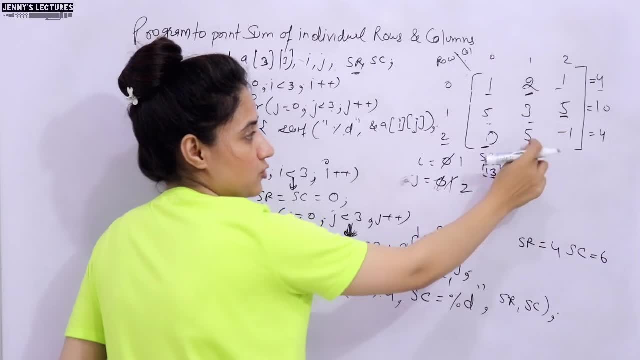 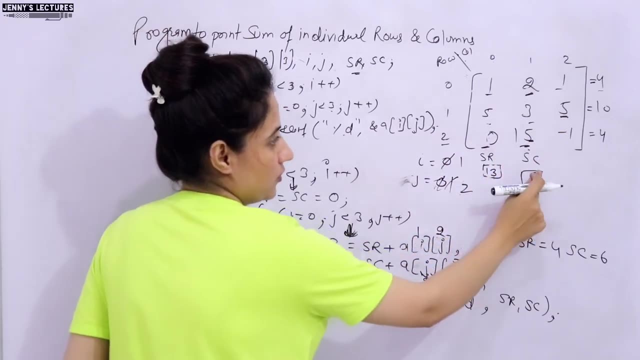 5 we are accessing, Although both value are same, but I am accessing this 5.. Let me change it. It is 15.. Suppose, Right, So now I am accessing this 15.. So 15 plus 5 is 20.. Right Now, J plus. 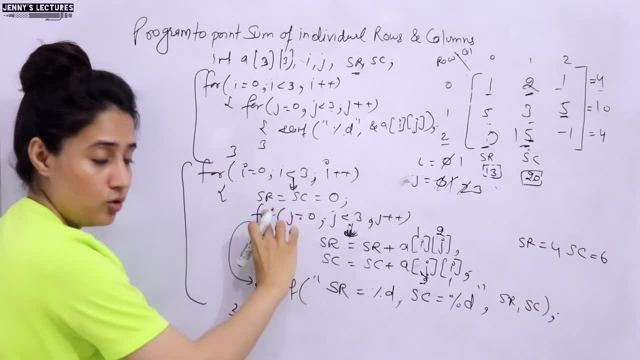 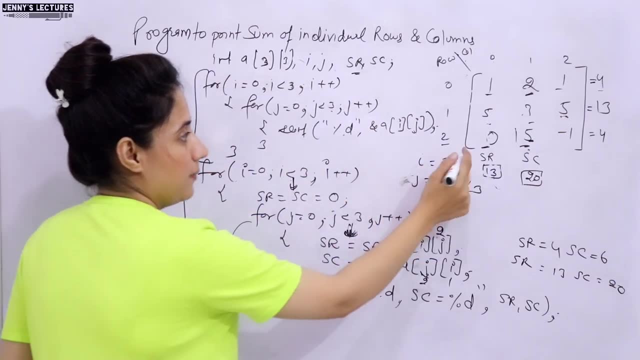 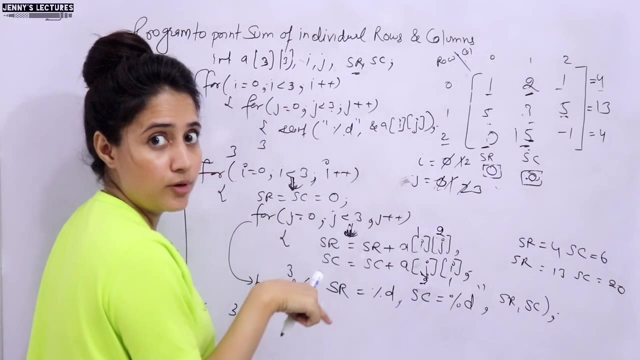 plus J becomes 3.. Condition is not true. And exit from the inner loop. And now again we will print SR equal to 13.. SC equal to 20.. Now again, I become 2.. Condition true: enter here. And again we are going to initialize it with 0 and 0. Because now we are going. 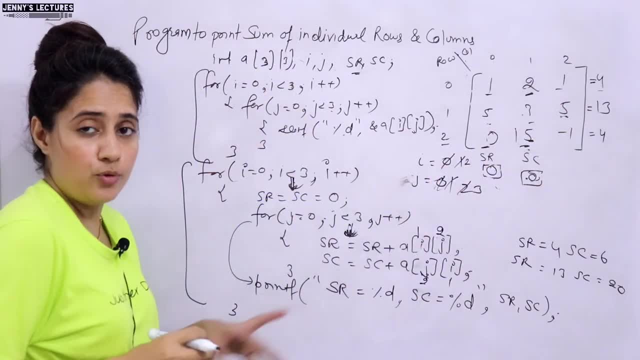 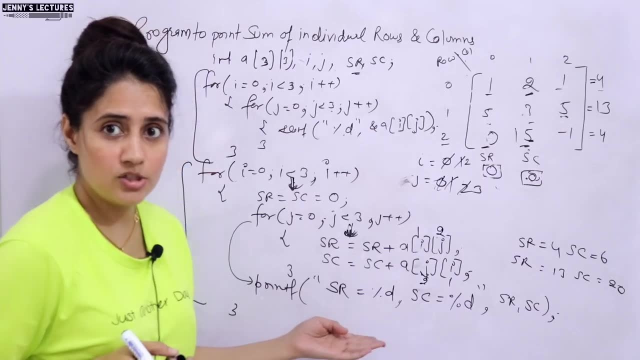 to calculate sum of third row and third column. I hope you can dry run this completely at your own Right. No need to complete it here. So I guess it is clear to you now The logic: How to do sum of individual rows and columns. 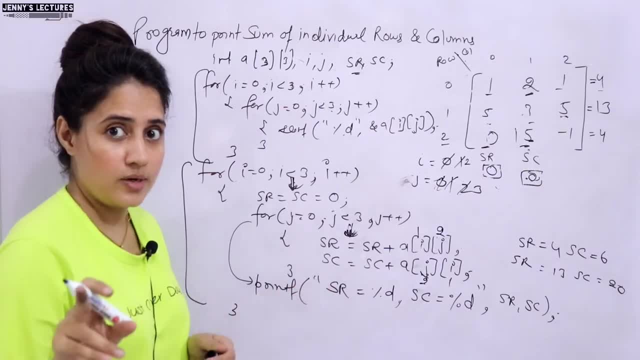 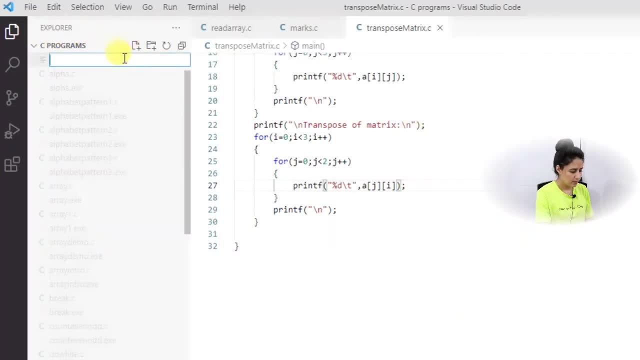 Right. So now let me just show you the output on my screen. Let me do the practical of this thing. So now let me create one more file for you, And I am just writing what Row, column sum dot C, Right. 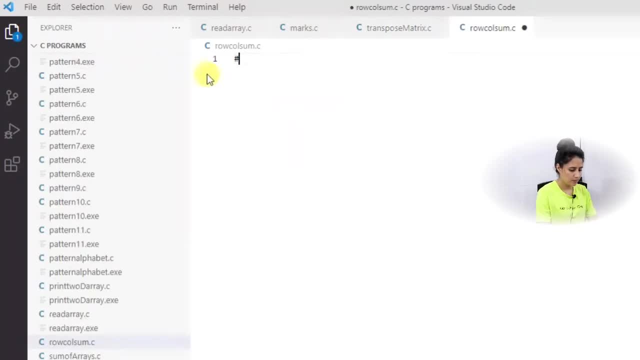 Right Now we will write main function and same. we will take an array of size 3 into 3 and i j some row I am taking and one is some column I am taking right. 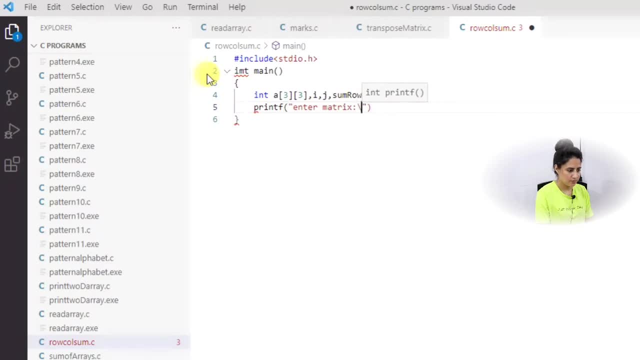 I am just writing here: enter matrix. and now I am just writing the logic to read the matrix Within this: we will use scanf. sorry, it should be address of a of i and j. right, and that is it Now what we will do. now we will do sum right. 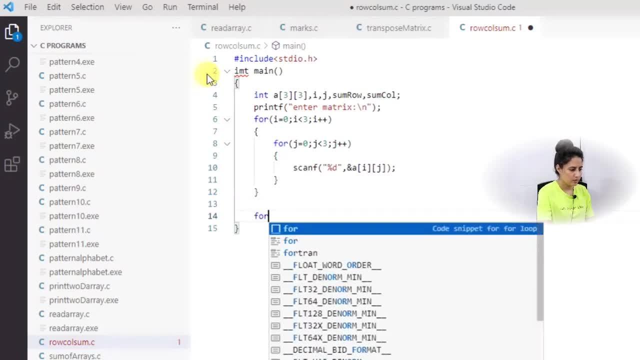 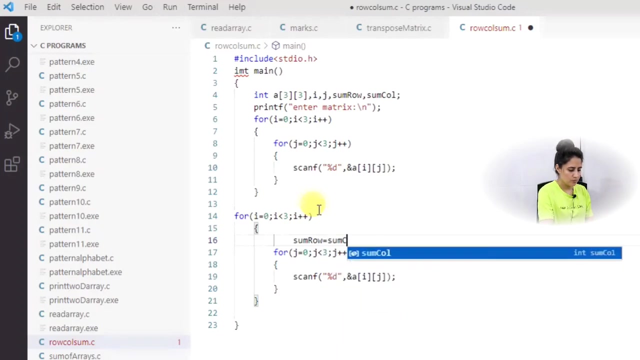 So now again, I am just copying the for loop from above. ok, So the condition would be same within this outer loop, we are going to what? initialize what? sum row equal to sum? Both would be 0, sum row and sum column. right Now i, j and here, rather than scanf what, just use the formula first of all, sum row plus. 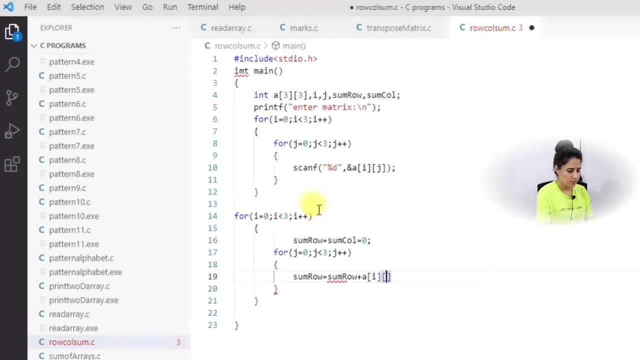 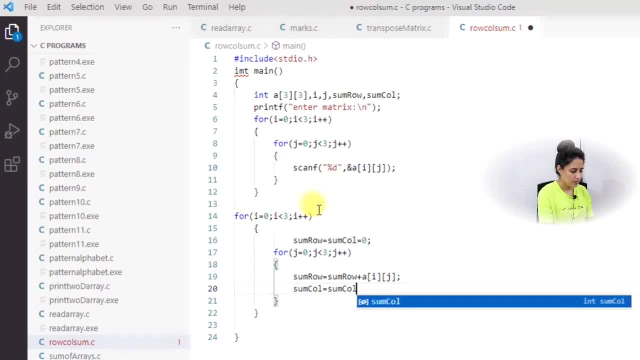 So I am taking i, j and here So i am taking a. well, that is enough. or I am taking a And one item number to finally How to take a number after Let. it is h 11.. So I am taking this id called As met in here. 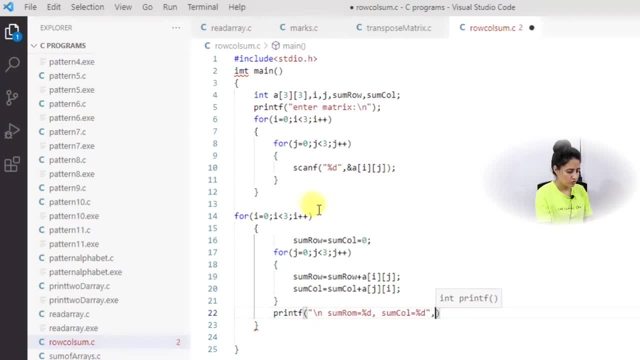 Now what I will do is I am taking all Same function. So 2 variable, 2 percentage d. first, percentage d will be replaced with whatever the value in some row, and second would be whatever the value in some column. variable right. 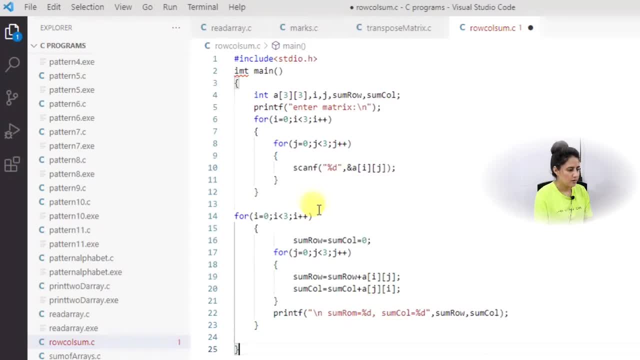 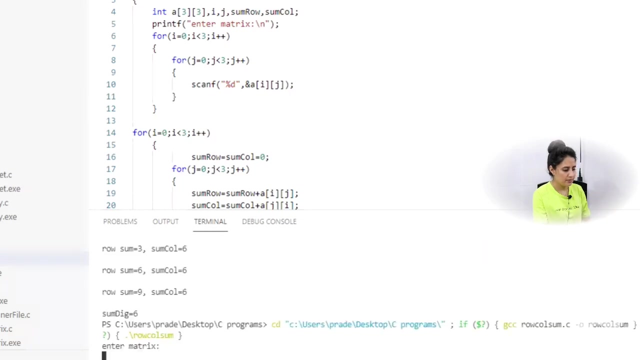 And I guess that is it. it should be int main, right, let me save it and now let me run it. I hope it will work. Say it is asking: enter matrix. so I am entering here what value: 1,, 2,, 2,, 2,. this is second.